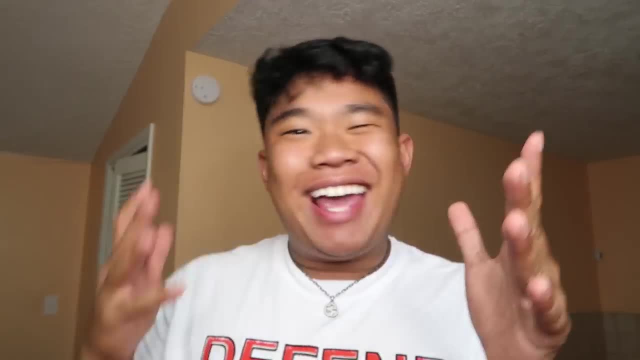 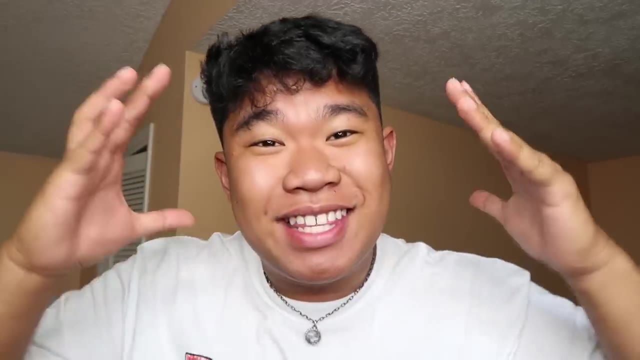 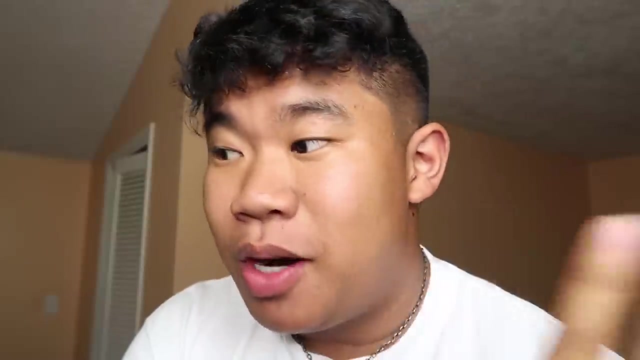 Hey, you know the vibe. what's going on, guys? on this magic, you're back at it again with another video. I hope all y'all are having a fantastic day. Thank you so much for taking time out of your day to watch this video today. We got something really special, dude, I swear. I say that for every video, like every video special, every video special when I'm with y'all. 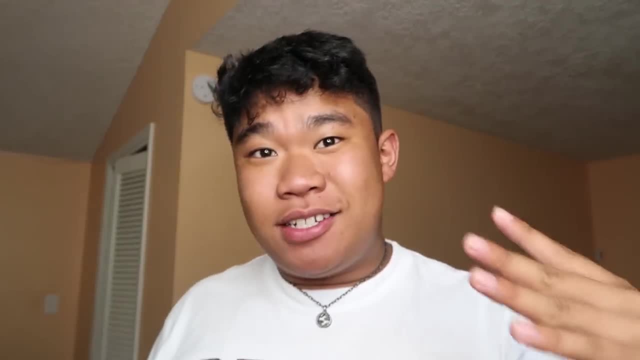 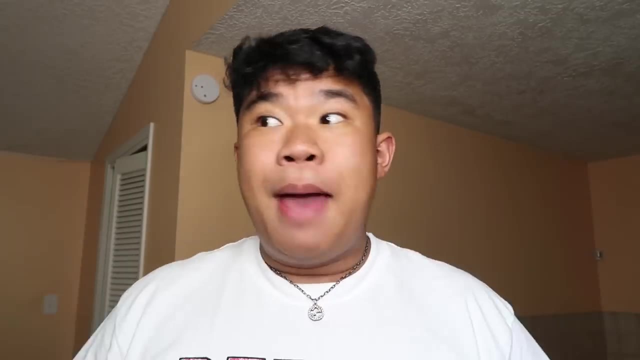 You know I'm saying Today we are teaching some card tricks. actually today We were teaching three card tricks. three, that's six. I could literally have no skill with a deck of cards and pick this up and start doing this in literally 5, 10, 15. 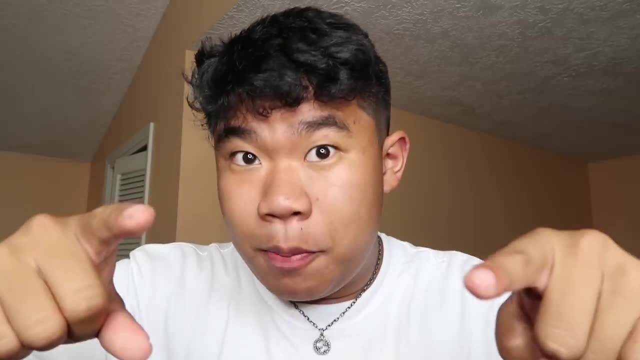 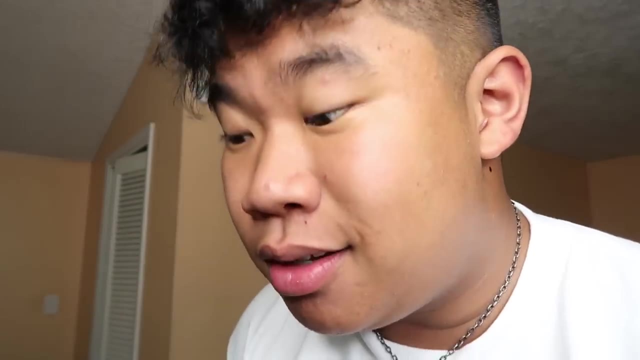 Maybe an hour, but it's not gonna take you very long to learn these card tricks. But real quick. before this video starts, if y'all are new to the channel, hit that subscribe button down below. I see a lot of new people watching this video and I better see y'all hit that subscribe button. I'm not kidding. 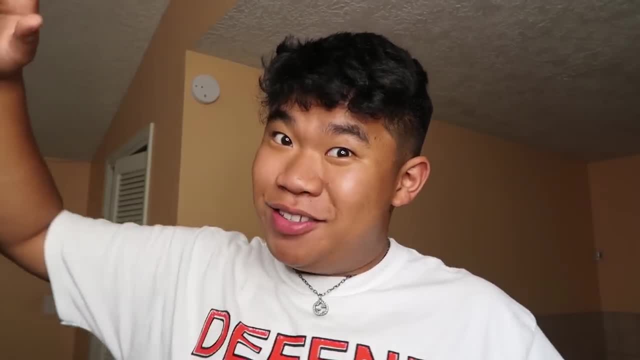 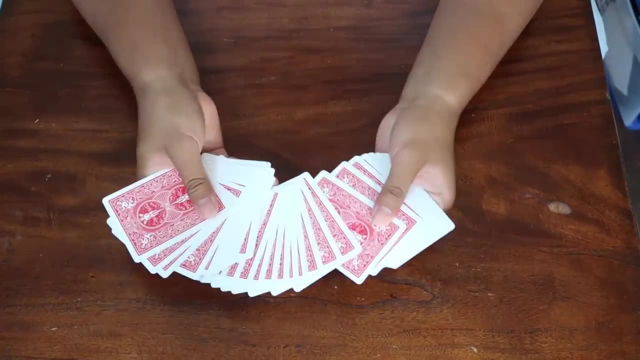 I'm watching you. I know where you live. with that being said, let's get right into the magic, alright. So I'm gonna first show you the performances of all of these magic tricks. again three really easy card tricks that y'all can do at Home right now. 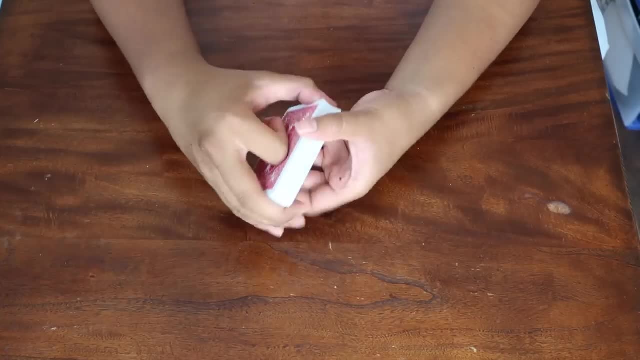 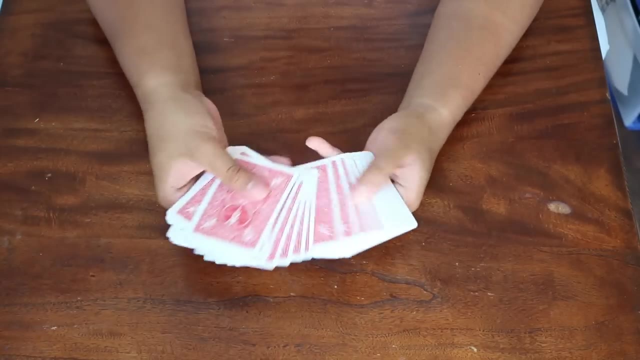 I'm gonna show you the performance and then I'll teach it to you. for all of these magic tricks, all you need is a Deck of cards, as you can see, and you can have it shuffled up and mixed as well. What I have the spectator do is I have the spectator pick any card that they want. so in this case, 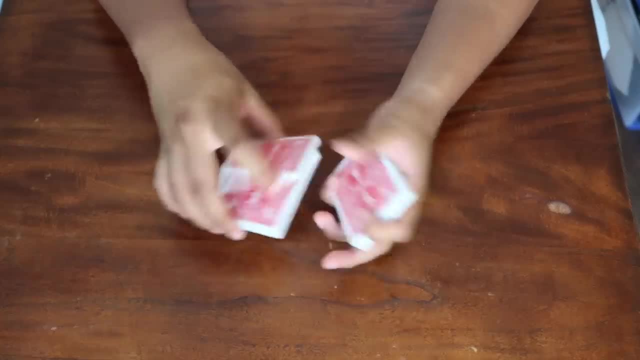 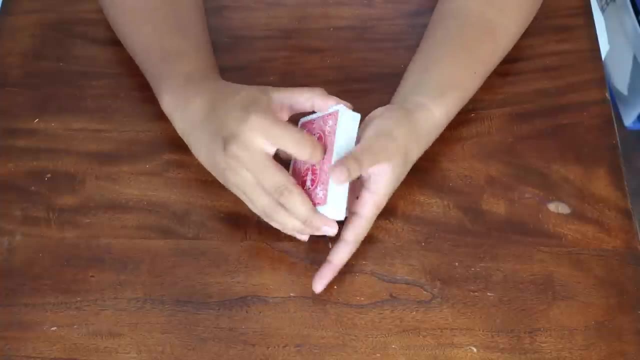 We got on the nine of diamonds. We're gonna take the nine and we're gonna lose it into the middle of the deck, Shuffle it up a little bit and you know, and even give it a nice little shuffle like: so now We're gonna grab a random card here, for example the, the jack of clubs. This is not your card, obviously. 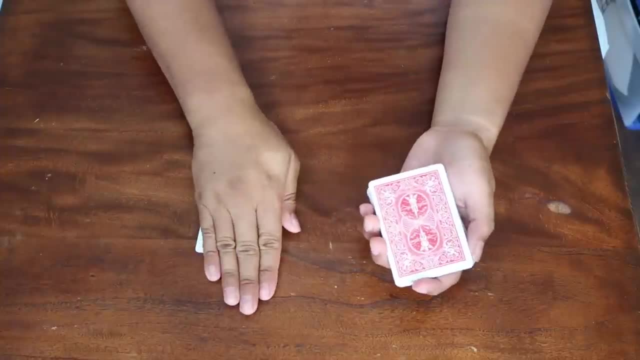 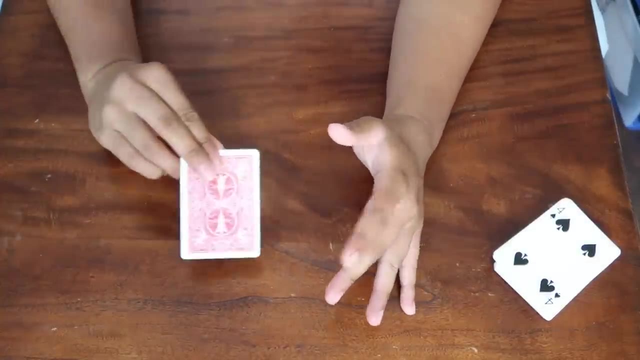 And? but what we're Gonna do is we're gonna set on the table and just place your hand right on top of that jack. all right, cool. now What we're gonna do is a little bit of magic, We snap our fingers and, just like that, that jack turns us into one card, and one card only the nine of diamonds. 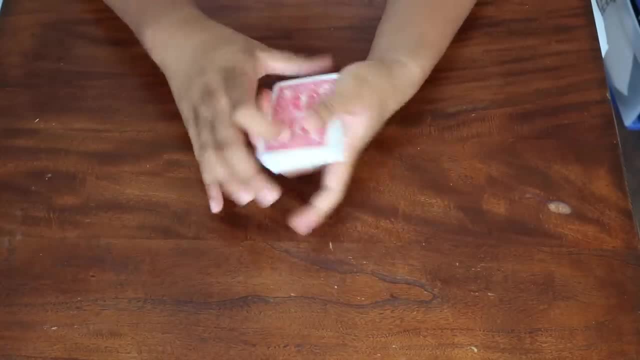 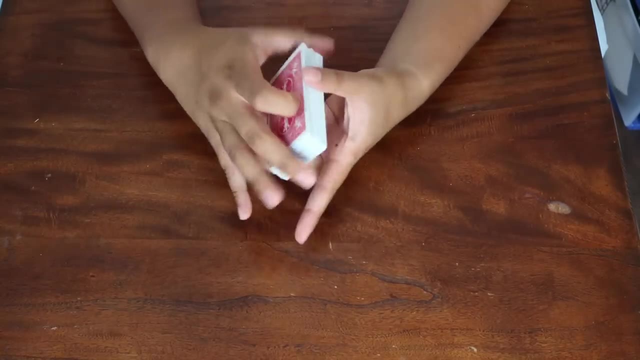 Your selected card. so that's the first card trick. Let's get into the second card trick. alright, So for this card trick, what I'm gonna need you to do is just go ahead, touch the back of any of these cards. So let's say this one right here. Let's take a look at what card you picked. you pick the, the six of diamonds. 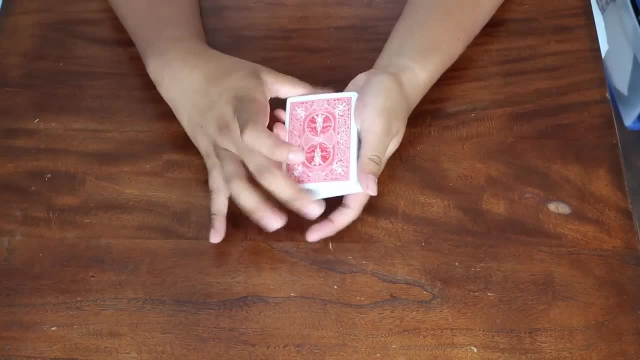 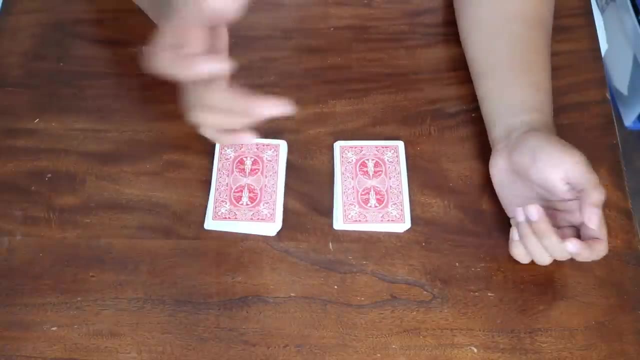 We're gonna take the six, we're gonna lose it roughly into the middle, Just like so, and that. what I need you to do is just cut the cards anywhere you want. a half way, a little more, a Little less, they go ahead, cut the cards And I'm gonna take the rest of the cards and we're gonna mark where you cut. now you could have picked any card, your card. 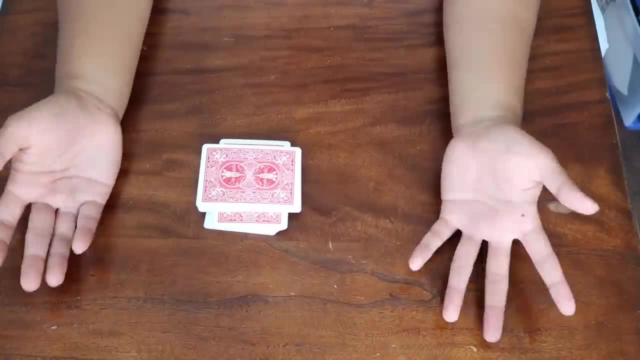 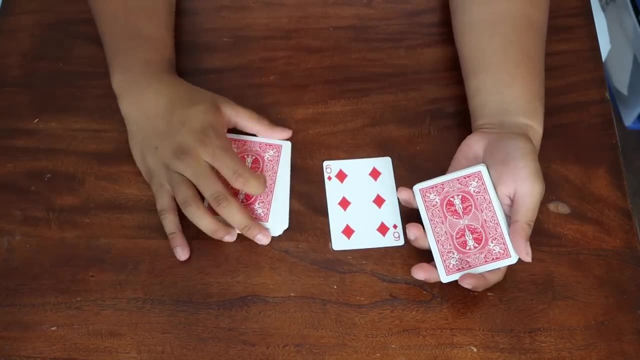 Is lost somewhere random in the middle of the deck. there are 52 cards in the deck, But somehow how did you cut perfectly to your card the six of diamonds, just like that? that one is really cool too, And we're gonna go into the last one and then I'll teach all of them for this last magic trick. 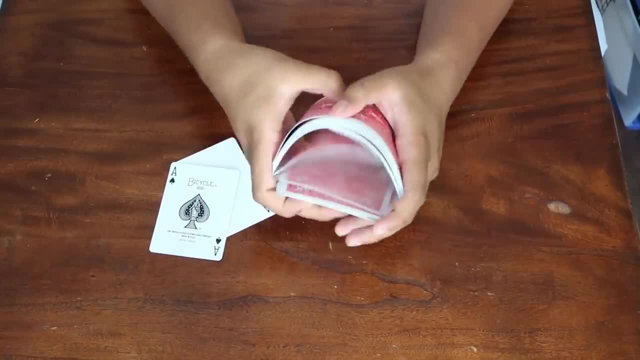 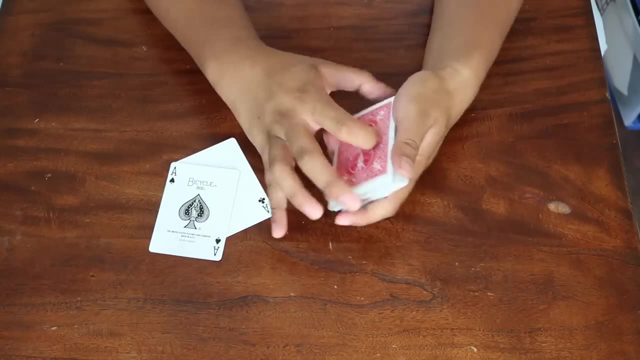 What we're gonna need are the two aces. what we're gonna do Is we're gonna have the card shuffled up and mixed and we're gonna have a card selected, for example, The jacket clubs. we're gonna take the Jack we're gonna lose into the middle of the deck. 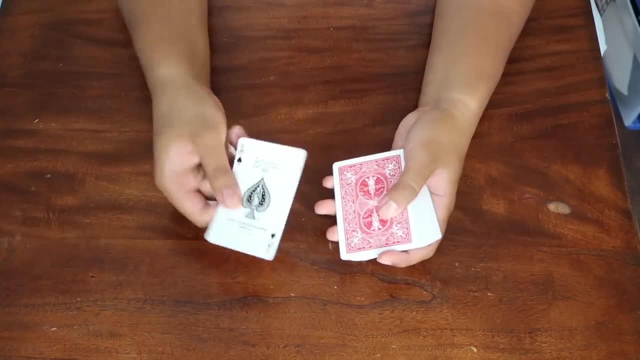 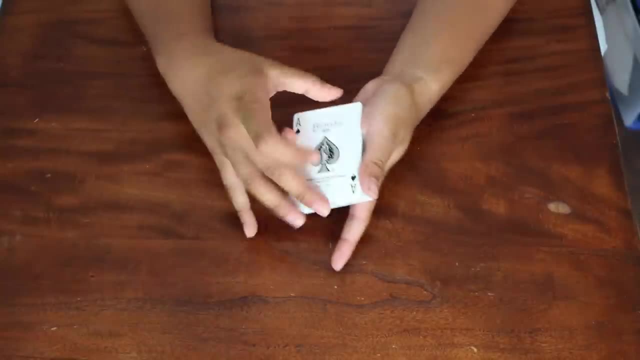 Shuffle it up a little bit and then we got the two aces here. Here's one ace right here, and then here is the second ace. um, like so we got both aces here. We're just gonna leave that on top of the deck and go ahead and cut the cards. 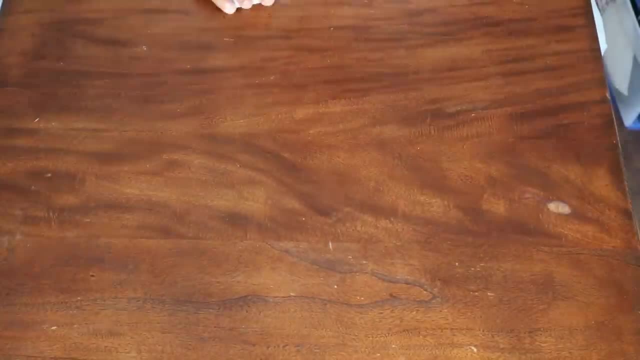 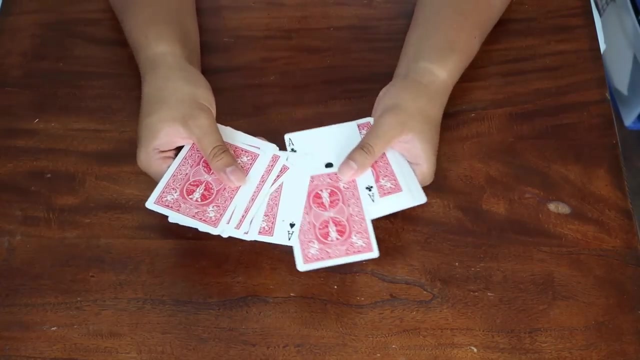 So they go ahead, take the cards, they give it a cut, they complete the cut And then you literally give it to them in their hands And you say: just snap and Just like that, when they spread it out, Spread through the cards. there'll be one card in between the two aces. look at that, it caught one card. 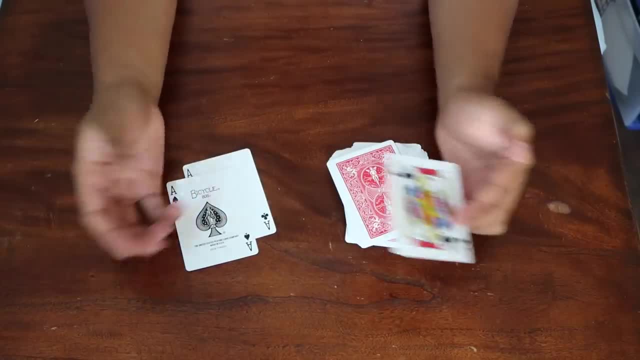 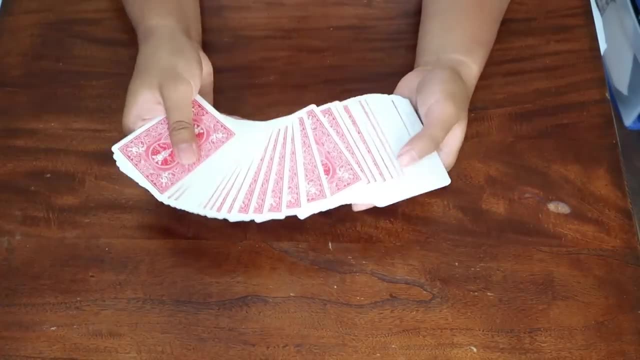 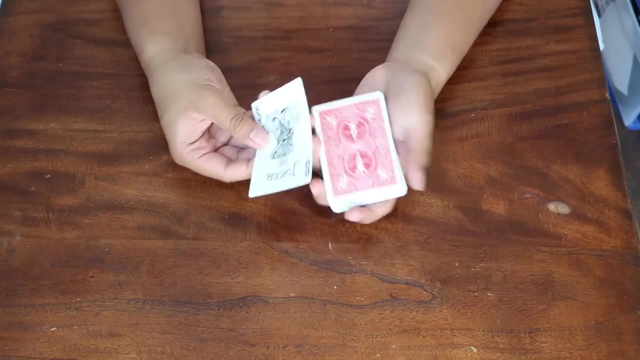 One card, only their card, the jack of clubs. all right, pretty cool. Three really cool card tricks that you can do at home right now. these will take very minimal practice, But it will take practice. so let's get into the explanation. The easiest one is the first one. you simply have someone pick a card so you start off with the Joker in this case. 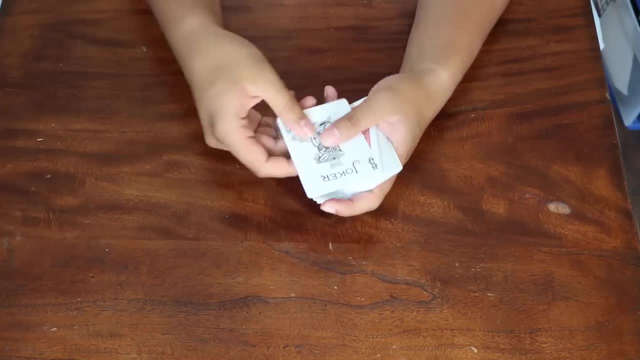 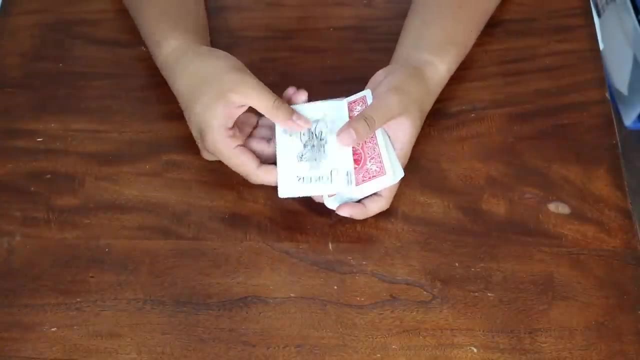 It's literally, honestly, a shovel deck of cards. It really doesn't matter. you have them. pick any card and what you're gonna Do is you're gonna Lose the Joker into the middle of the deck, but in reality it's gonna stay in the top. how I do this is I give the 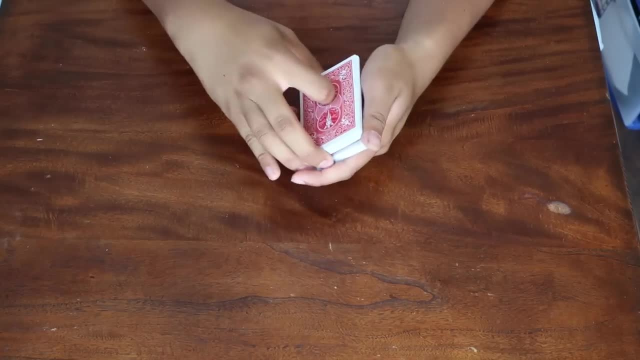 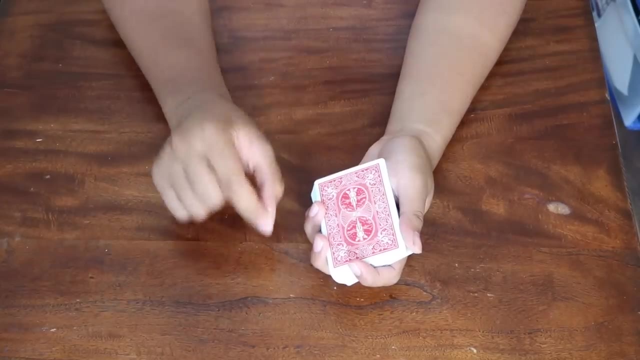 Cards a cut, so I literally like, cut the cards like so, and instead of completing the cut like so, I insert my pinky. as you can See, my pinky goes right there and this is what it's called a pinky break. I'll leave a link at the top of the description on how you can do a pinky break. 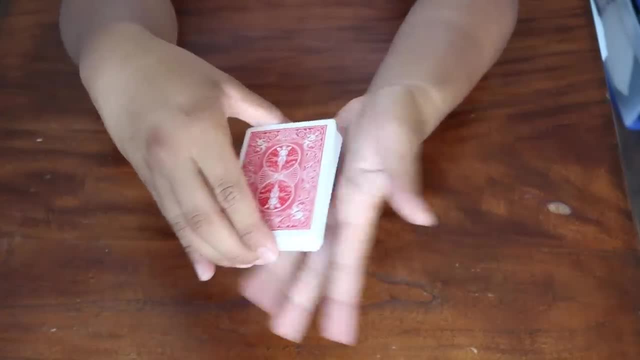 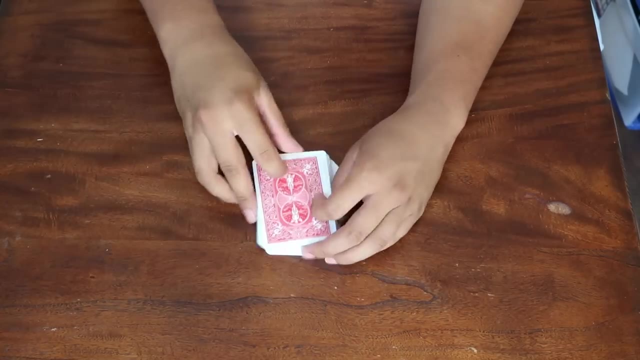 But the simple concept is this: we're gonna take the cards. We're gonna get half of the cards into my other hand. you can literally do this on the table. if you don't want to do It one-handed, so say their card is on top, they have the Joker, okay. 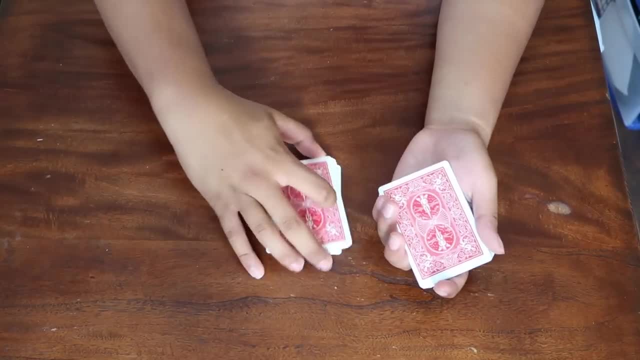 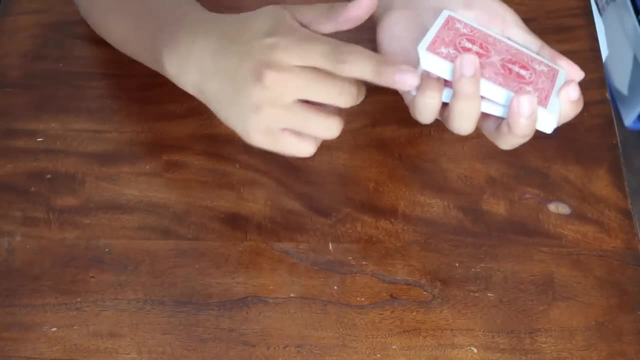 And you say, hey, We're gonna mix the Joker into the middle, take half the cards put right here, And then we'll take the other cards and we'll put it on top. now, when you put it on top, You're literally just gonna put your pinky right there to hold a little break, like so. so now you got a break and to go. 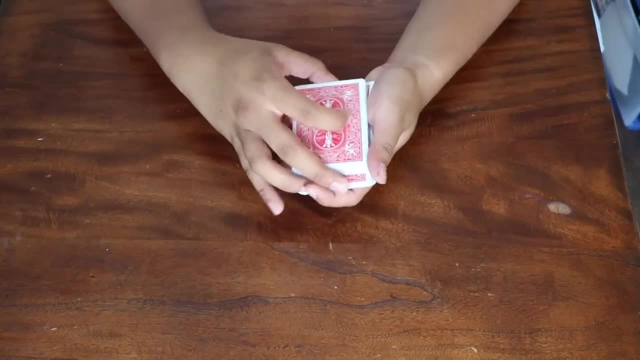 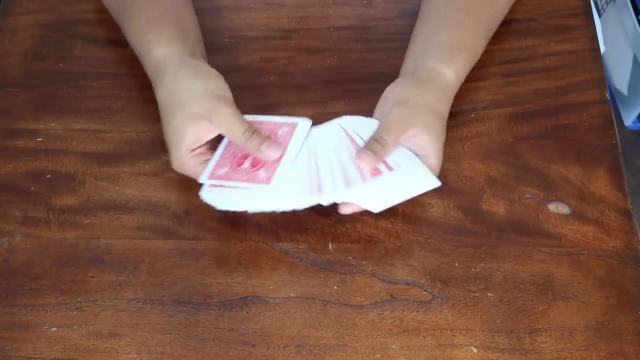 Back to where it was, where that this card is on top wherever the break is, you literally just lift from that break. So you just lift from the break and then you give it another cut and all in all it would look like this: They pick a random card, for example the two hearts. you say, okay, watch the two. 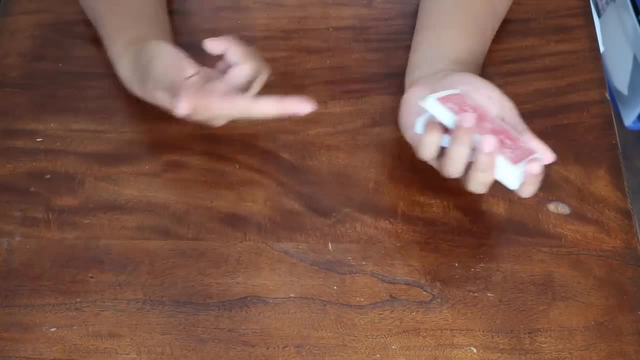 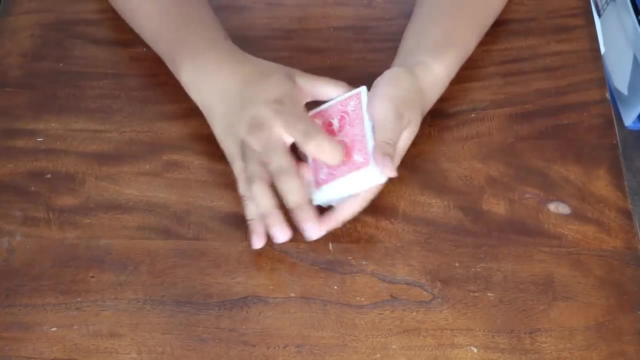 We're gonna lose into the middle of the deck by cutting it and lose It to the middle, and then you got the break right there. You just answer your pinky, you say, okay, We're gonna give it a few more cuts, Like so. and then you can literally keep repeating the same process. 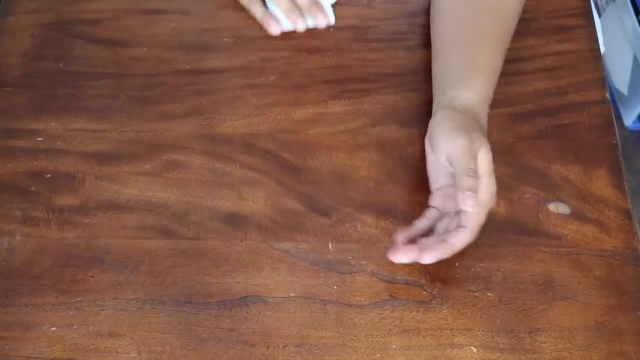 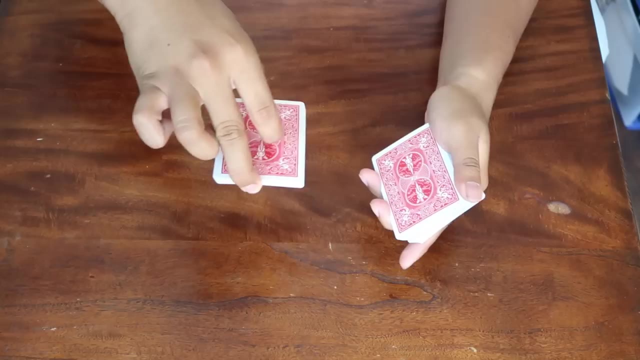 of Cutting the cards and then putting it back in order. if you're more advanced, you can do this where it's like this, and then you Can grab- not exactly from the break below, less than, and then the whole break, Just like. so, whatever you want to do- to lose a card into the middle of the deck. 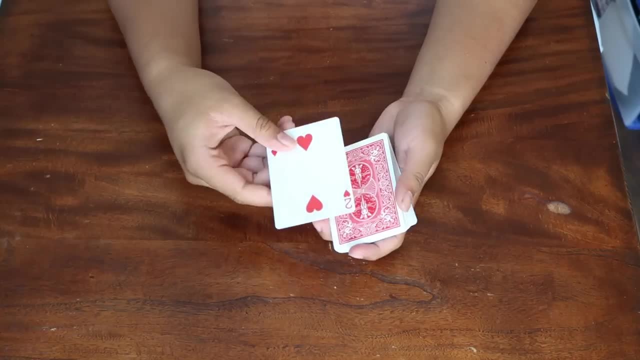 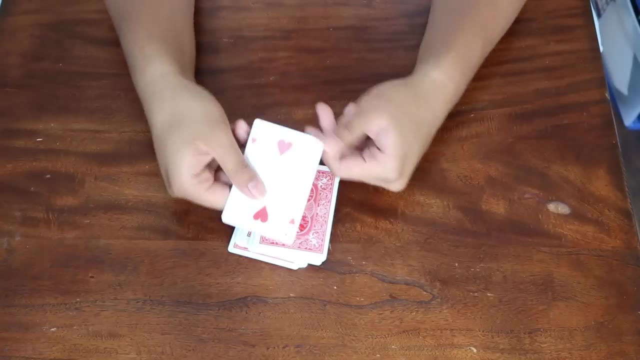 But in reality, will stay on top. there's so many ways you can do that to control the card on the top. Whatever you want to use, I'm just showing you the simplest way, Which is simply losing it and then cutting it back, like so, once the cards on top. 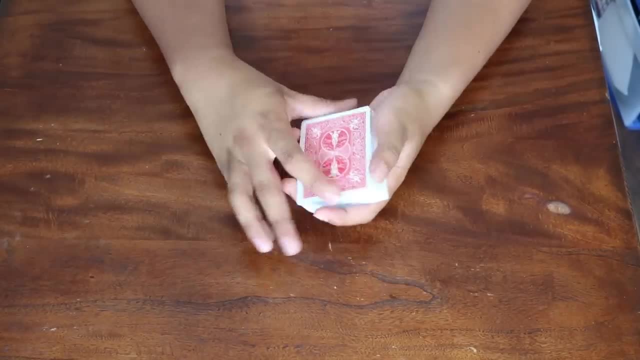 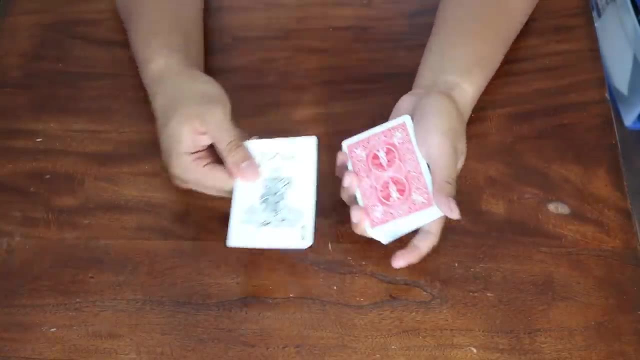 You're gonna need to do a move called the double lift. such an easy move. All you're gonna do is you're gonna take two cards and you're gonna lift them at the same time to reveal as one. That's a double lift. right there, It may look like one card. 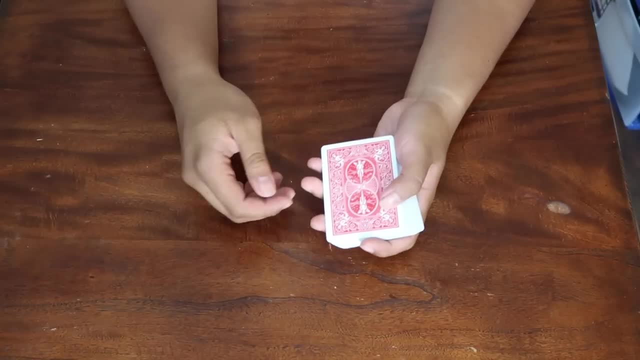 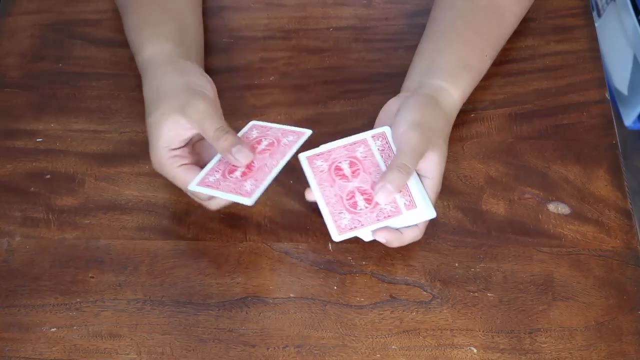 But I'm holding two to do this. how I do this? at least there's two ways. the easier way would literally be like: okay, So your card is lost somewhere in the middle of the deck. I pick up two cards. while I'm saying that, I Literally just pick up two cards. so your card is lost somewhere in the middle of the deck. 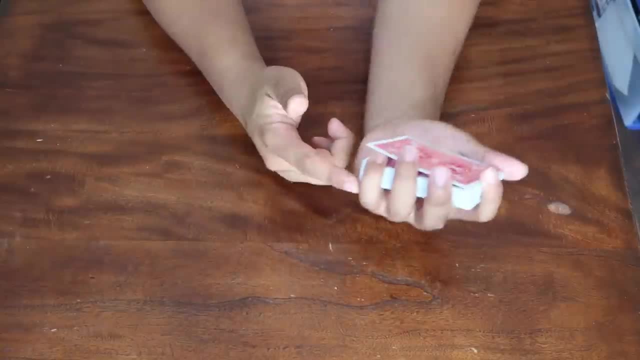 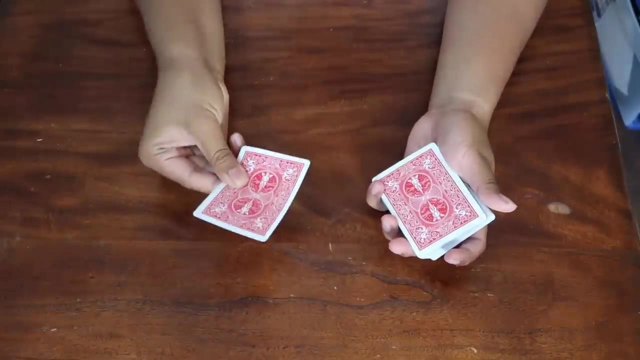 I'm holding two cards. you insert your pinky and you place the rest of the cards on top, like so, and now you have a Little break and you can literally just lift those two cards at once and show a card. It looks like I'm holding one card, but in reality it's two. a more advanced way: is this thing called a wrist kill? 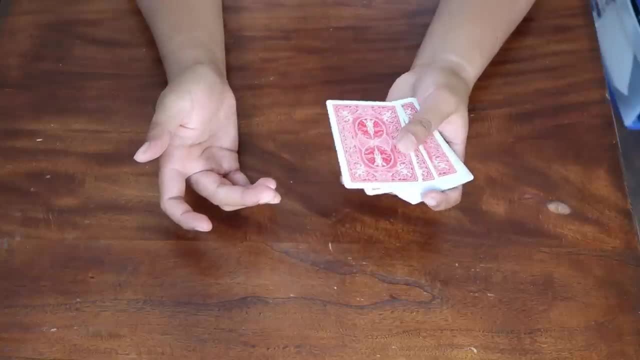 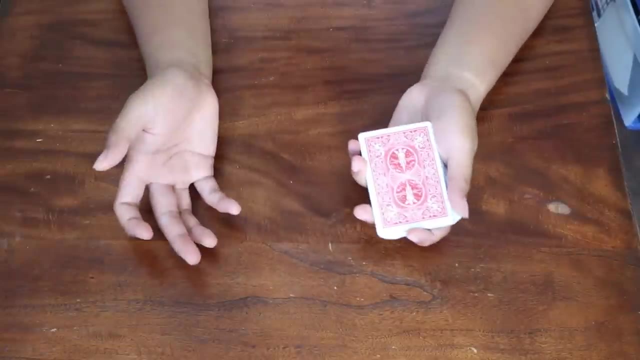 It's when you push two cards with your thumb and then you pull it back in Inserting your pinky. this is all done one-handed. It looks something like this: literally just like that, but you do that while you're turning your wrist. You literally just go like this and then they won't see the action any way. 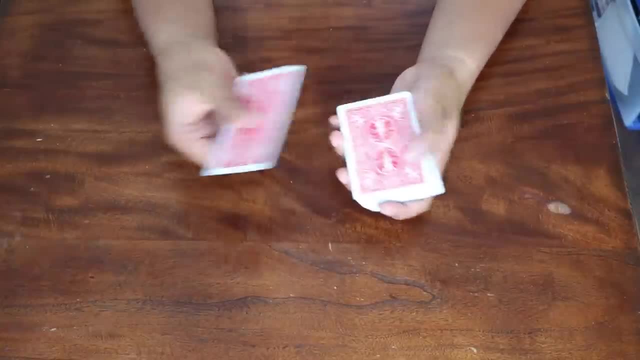 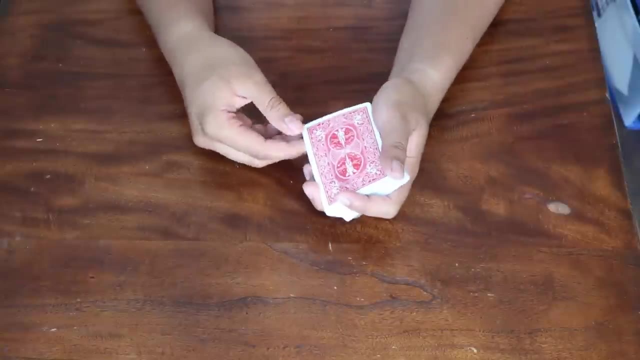 You want to do to get your double lift. the easiest way again is literally just go: okay, your cards lost somewhere in the deck. You have two cards in your hand And you enter your pinky and you place the two cards above your pinky and now all you do is you lift two cards at 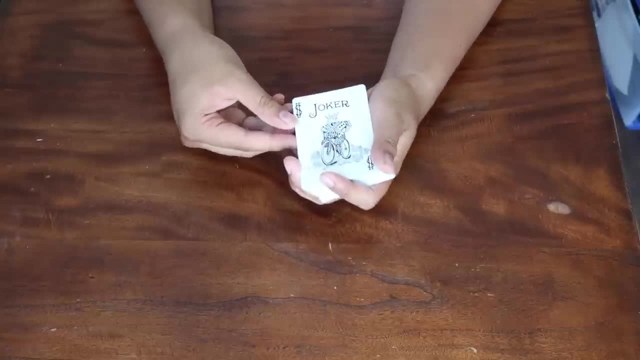 Once there you go, That's literally it. you say, okay, This is not your card the Joker. okay, cool, We're gonna take it, We're gonna set that Joker down. but in reality, This is the two the Joker's in the second spot. 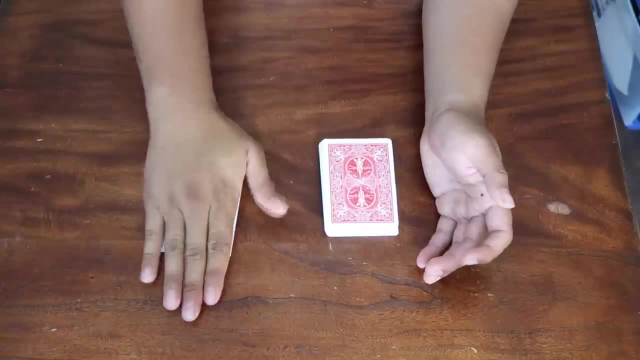 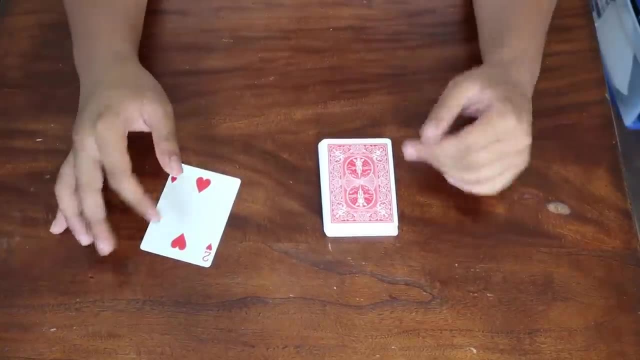 They think this is the Joker. though you set it down, you say, hey, We're gonna place your hand on top. You snap, and now it magically changes into their card. pretty easy, to be honest. It will take a little bit of practice, but again, This is such an easy magic trick. 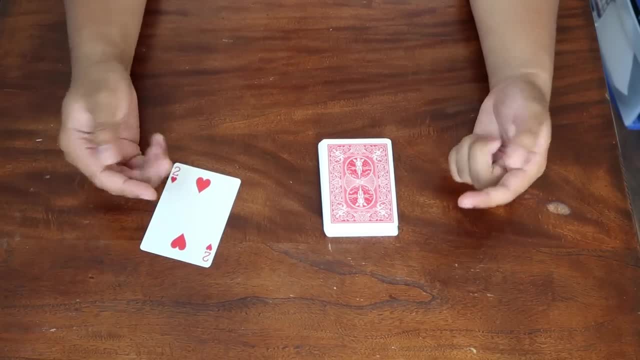 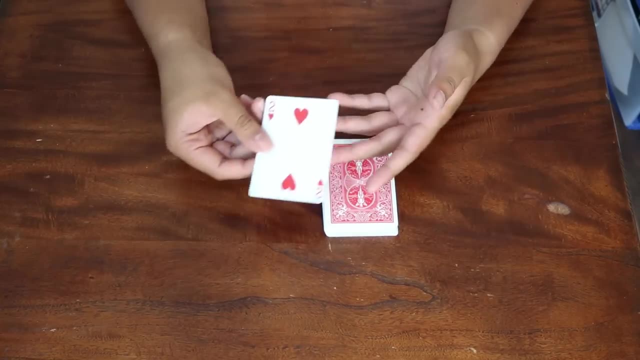 It will take a little bit of practice, but again, It is so easy and once you get it down, you really got it down and you will blow minds. I use this trick till this day and it's one of my go-to effects, So I really recommend you check it out and really practice this one. the second card trick. 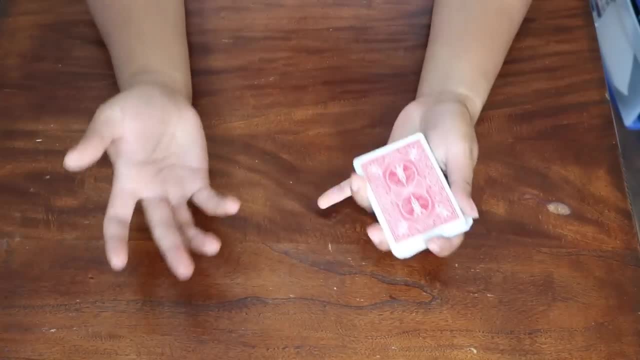 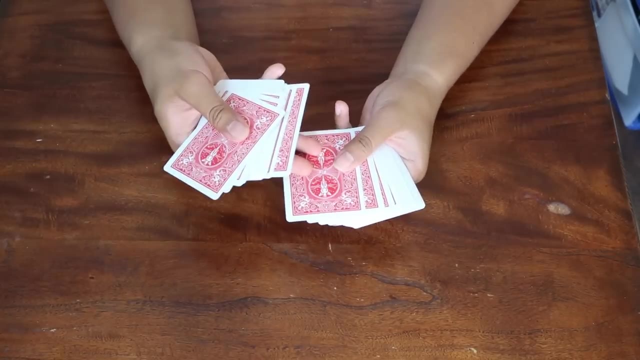 I'm gonna teach you is literally. I would even argue that. say that this is even easier And it uses the same concept. so you have a shuffle deck of cards. You have them Point to any cards. so say, they point to this card right here. you say okay, you bring it to the top and 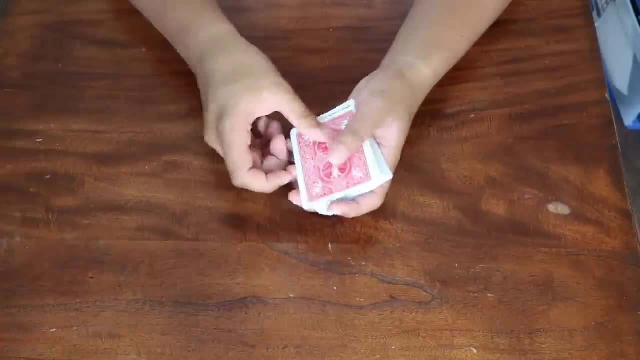 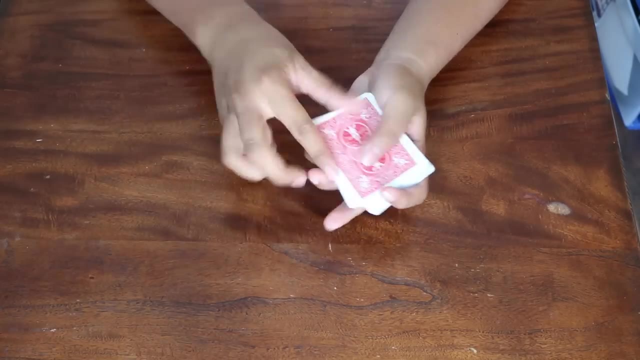 You're just gonna do a double lift. you literally are gonna lift two cards. You can get it set up by saying, okay, You could have picked any of these cards, but you pick this one right here. and in that motion I was able to get that double on that little pinky under the two cards. 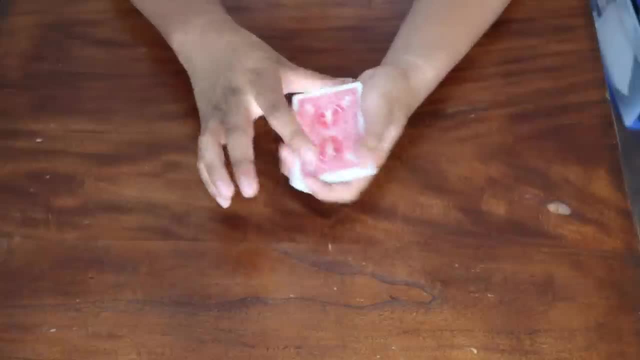 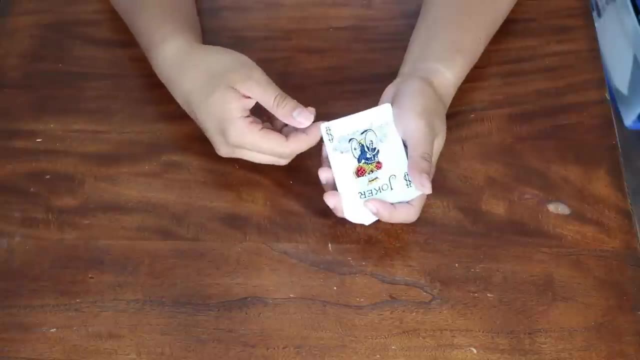 You can also just do this, whatever you want to do, to try to get a double lift, But all you're gonna do is whatever card they point to. you're gonna do a double lift. in this case is the Joker again, I don't know what the odds are of that, but we got the Joker. 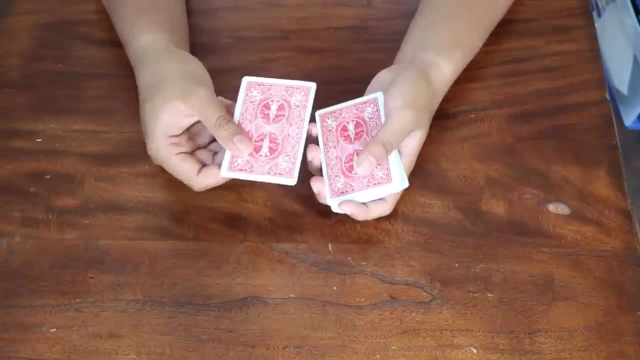 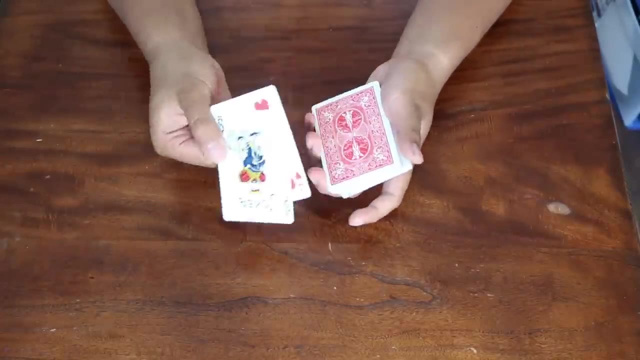 And then what you're gonna do is you're gonna say, hey, we're gonna take that card. They think this is the card, but reality this is the fake because again, you lifted two cards at once. They think that what you're holding right now is the Joker, but in reality This is the four. you say we're gonna take the Joker. 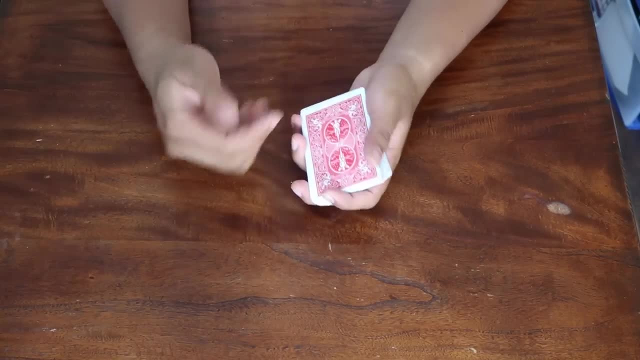 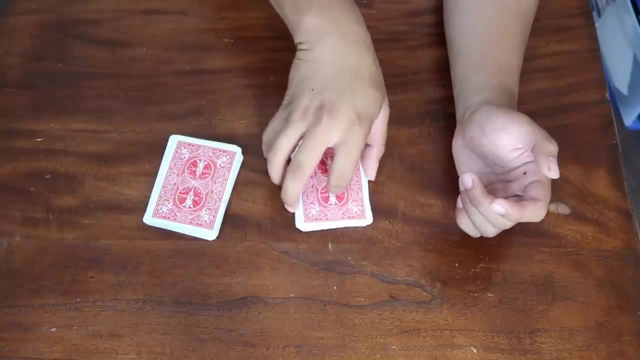 We're gonna lose into the middle again. We're not losing it to the mill because the Joker is still on top. and then you get into this little routine where you say: cut Anywhere you want, they cut the cards and you say, hey, we're gonna complete the cut. 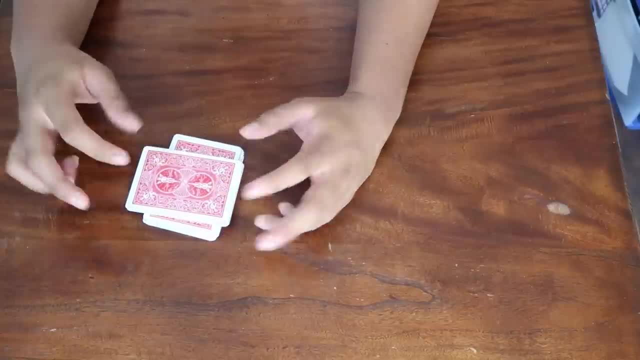 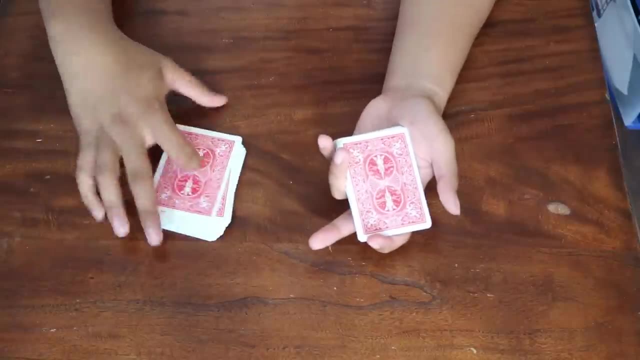 You're gonna take the rest of the cards and you're gonna make a little cross on Top of where they cut. now they're gonna think that they cut right here, but they didn't. this is actually the top card. This is the Joker, what they picked again. 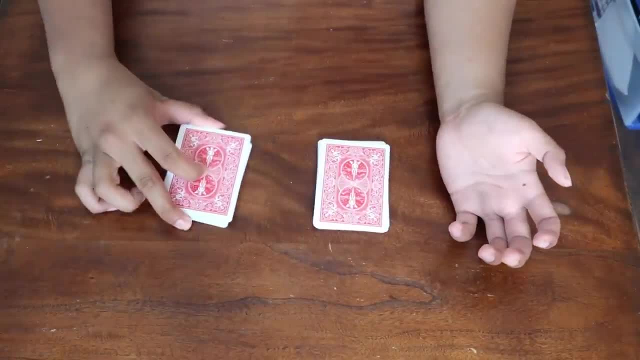 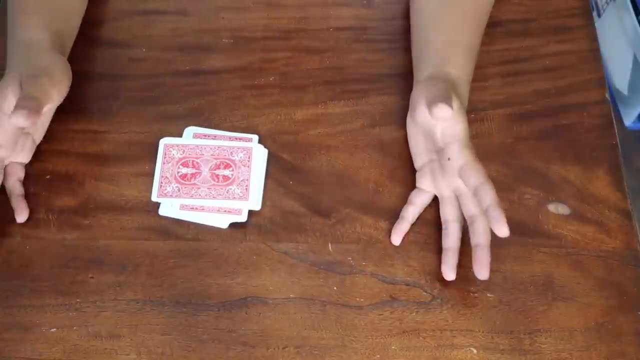 The Joker is on top. you tell them: cut anywhere you want, and you're gonna make it seem like they cut right here by taking The packet and going like this. Literally just do this and you start talking about the deck and then you go back to say, hey, 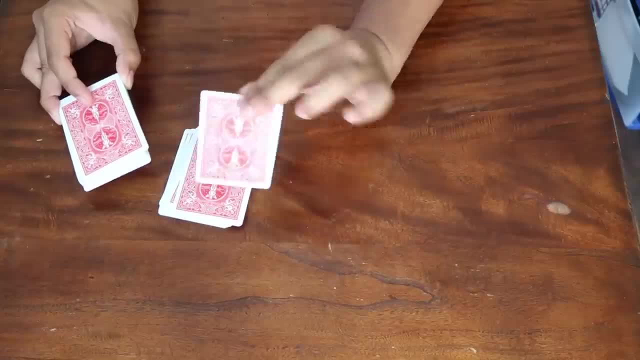 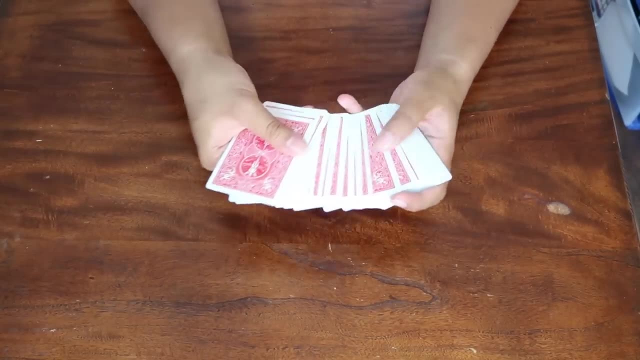 Let's look at where you cut to. they're not gonna think twice, They're gonna think they cut right here and is their card the Joker? I feel like I rushed through this one a little bit, So I'm gonna quickly go through it again. The total thing is they touch the back of one of these cards like this one right here. 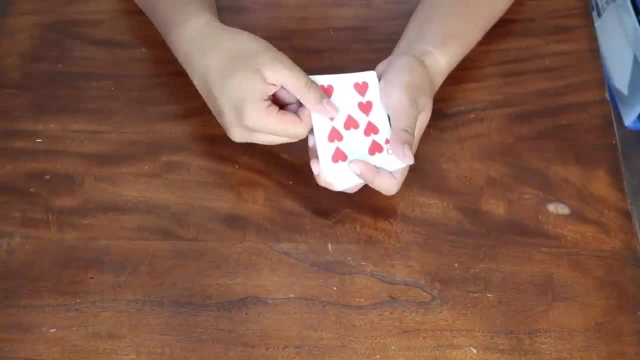 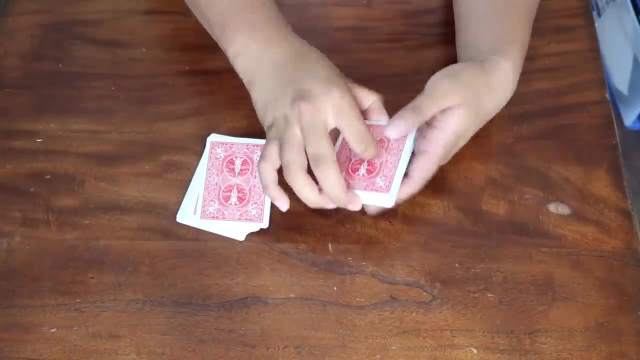 You do a double lift, you say okay, so in this case you pick the nine of hearts. We're gonna take the nine, which is not the nine is really the ace We're gonna lose into the middle of the deck. Cut anywhere you want. Okay, cool, We're gonna mark where you cut again. You're just placing it right on top of the top card. 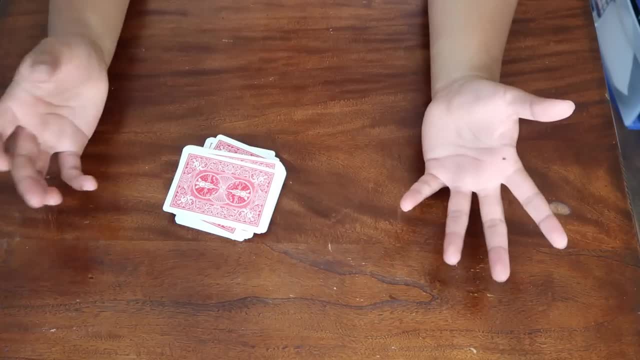 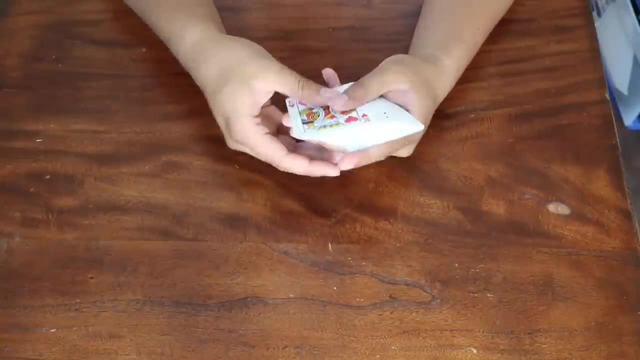 It's not really where they marked. You put it right there and then you say you could have cut anywhere you want, But you cut right on your card the nine of hearts for the last one. This is gonna be the hardest one of them all, But it is still. 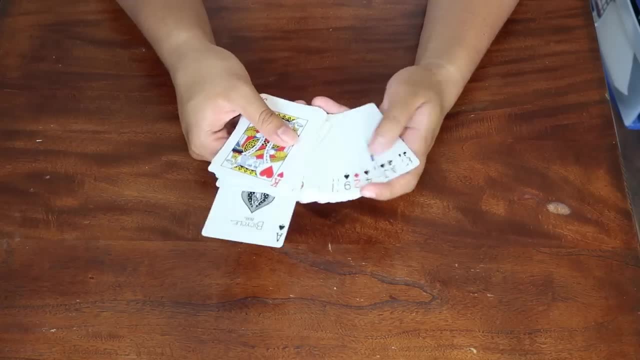 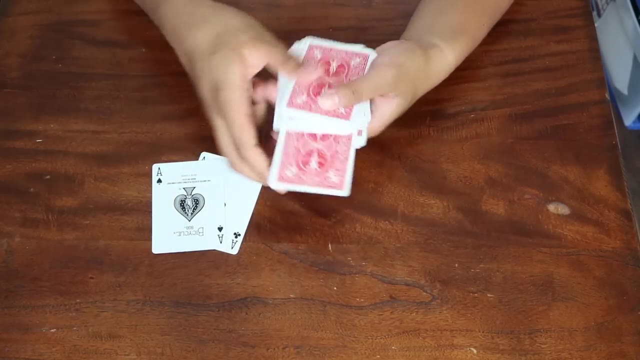 Not that difficult. so for this you're gonna need the two aces- Here's one, Here's two- And you're gonna say: hey, We're gonna use these aces to help me with the magic trick. What you're gonna do is you're gonna have them select any card that they want. in this case, 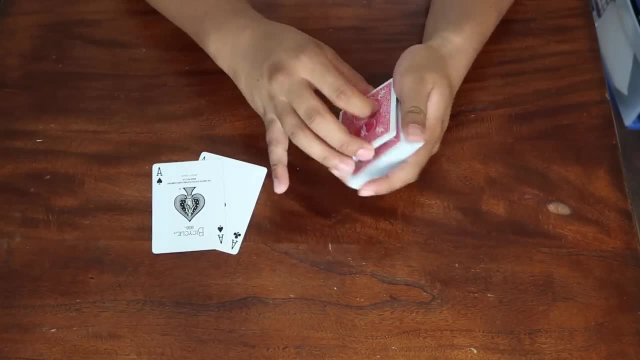 They got the two of spades. you're gonna lose it into the middle of the deck, But you're really not losing it just like the first trick, You just want to keep that card on top. However, you want to do that again. You can mix it up. 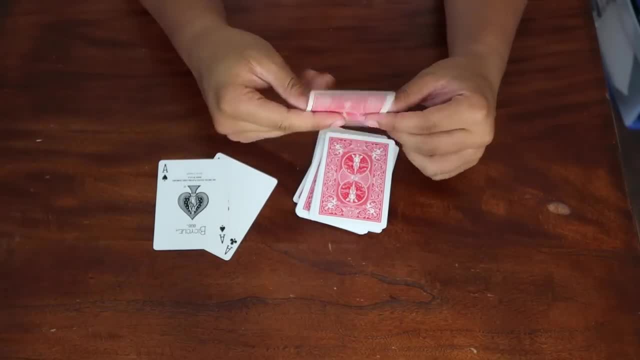 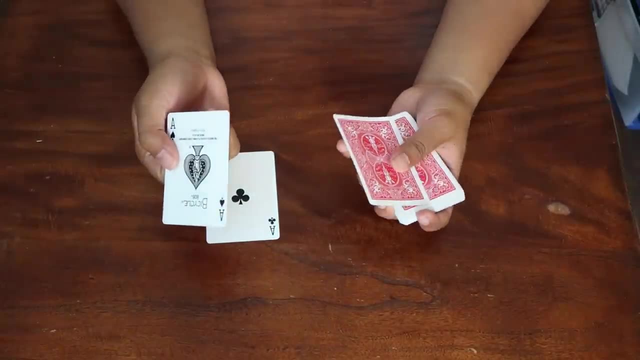 Do false shuffles, false mixes, as long as you can keep the two on top and convince them that it's lost. So the two is on top, But they think it's lost and you're gonna grab one of the aces and what you're gonna do is you're gonna need to get a break. 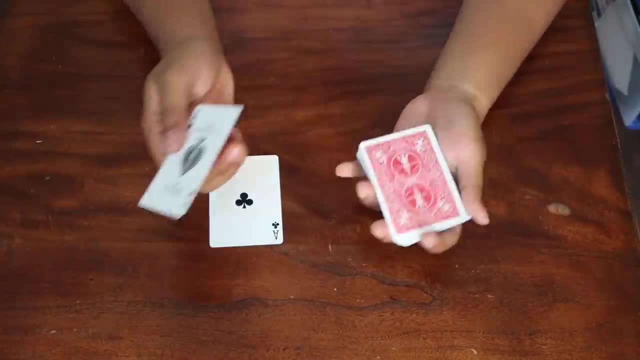 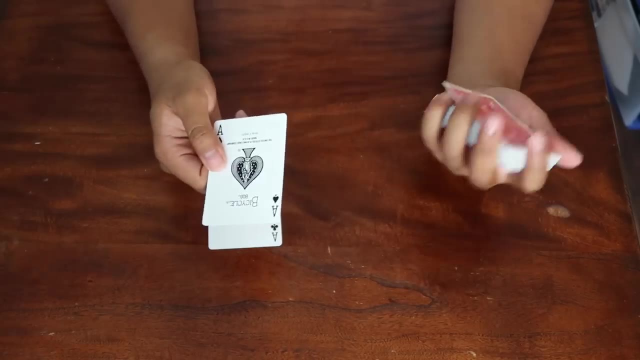 Under the top card. So, as you can see, I have a break Under the top card. how I did that is I literally pushed off one card and then when I bring it back in, I just insert My pinky like that. So now you have a break under the top card, You're gonna take the ace. 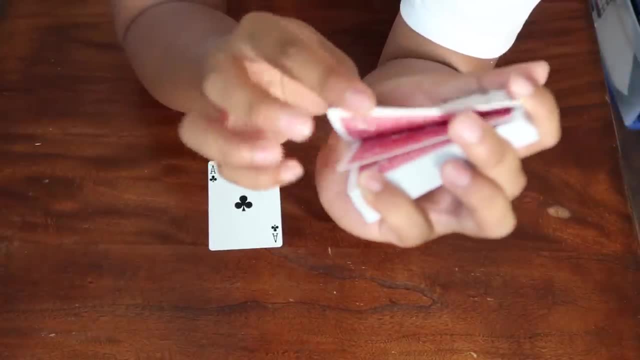 You're gonna place on top and now you have a little double break right here. It's like it's like the double lift, except back-to-back. So we got the two, we got the ace right there and literally all you're gonna do is, once you're in this position,